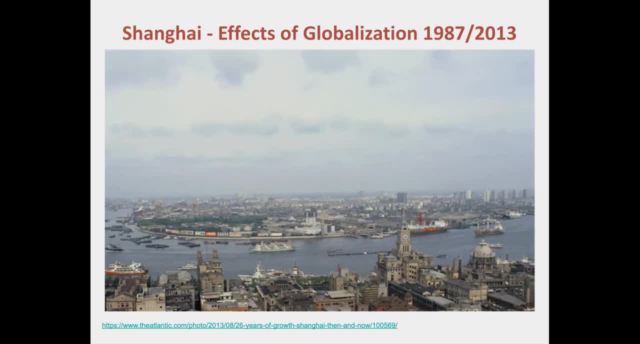 first of all, I wanted to show you this really cool gif that I found that shows Shanghai over the course of about 30 years. a little, yeah, a little over 30 years from 1987, which gosh, if you can believe it, I was a sophomore in high school all the way up to 2013.. And you, 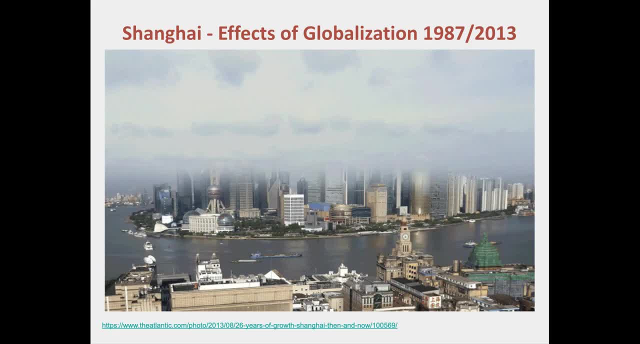 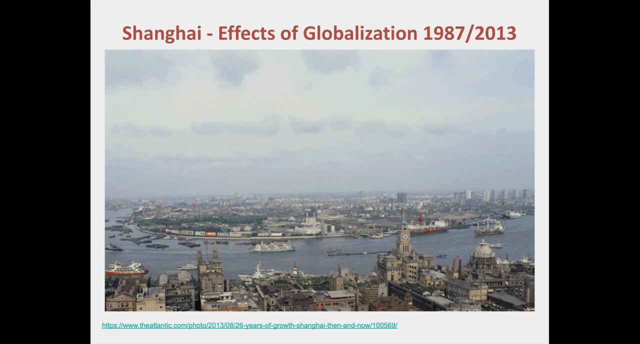 could see the difference here, And if I were to try and say, hey, what's the main idea of this particular gif? What I would say is: this is the impact of globalization, and nowhere can you see this more definitively than in Shanghai. So I'm going to show you a little bit of that. 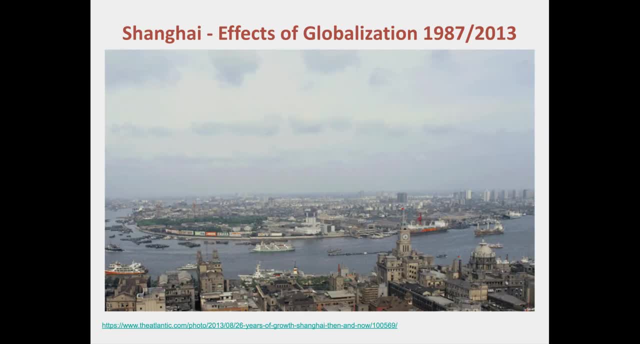 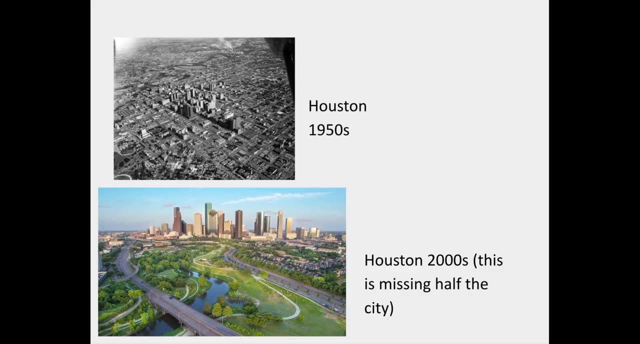 Some place like Shanghai, which is just totally due to massive foreign investment and trade with China. So here are two images of Houston in 1950s and then Houston in the 2000s- And I couldn't find a date for this particular photograph- And, of course, those of you that live in Houston, you 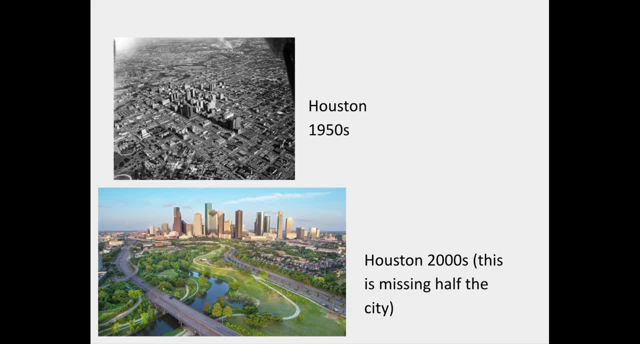 know that this is only about half of the cities. Houston has actually several areas that we don't necessarily consider them downtown, but this is the CBD, downtown proper of Houston, And then of course there's a whole other area of downtown And then of course there's a whole other area. 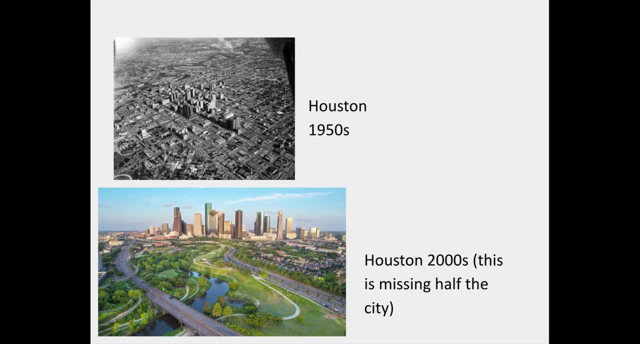 of downtown, And then of course there's a whole other area of downtown, And then of course there's a whole other area by the Galleria, which has just as many high rises, maybe some more high rises than this, But once again you could see just the incredible transformation over the course of 50. 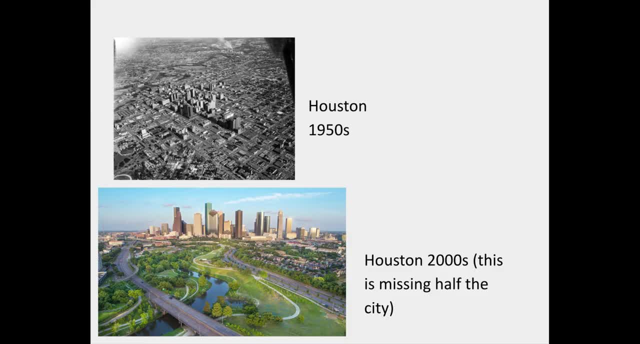 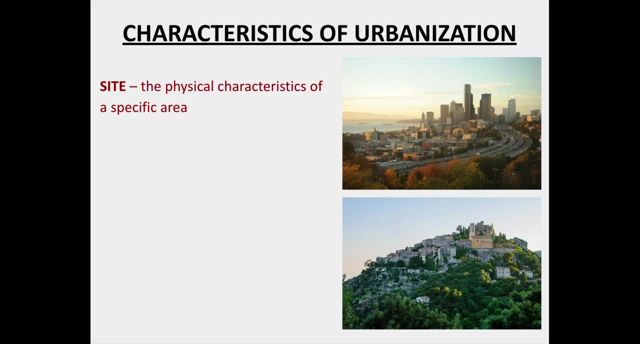 years. I know 50 years sounds like an awful lot, but really, over the course of civilizations it's just a blink of an eye. So today we're going to be discussing several different issues. The first I just want to discuss basic vocab. Sight and situation are terms that you learned back in 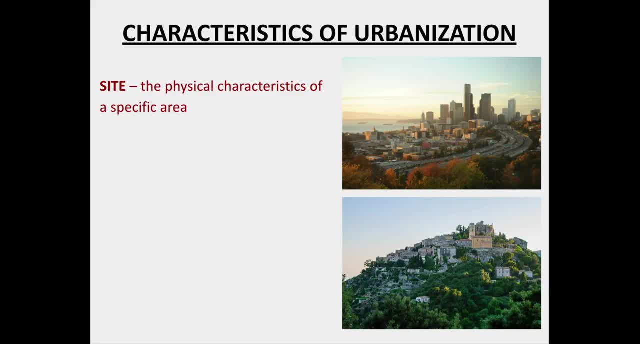 Unit 1.. And here they are again back in Unit 7.. Sight, if you recall, this is the physical characteristics of a place, So it could be like, of course, I'm in Houston. So Houston is an area that's incredibly humid and it's flat. It's not mountainous at all, It's almost coastal. We're close enough to the coast where we can consider ourselves coastal. It definitely impacts our environment and our weather here. So when you're looking at where cities were founded the earliest, 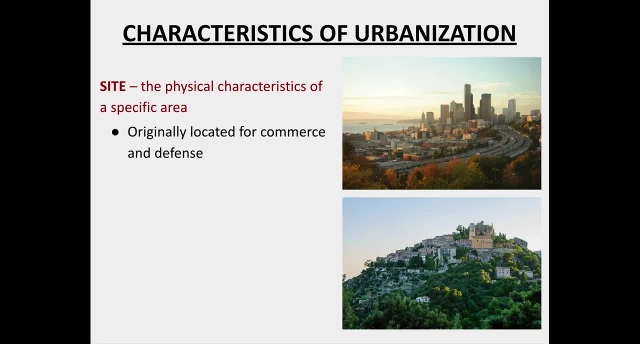 cities were founded in the late 20th, So places like Houston are going to be in locations that are great for trade and also for defense. You're going to want a location that's easy to defend, So, for instance, peninsulas could be great for this. Islands, of course, are super easy because you have your basic defense. 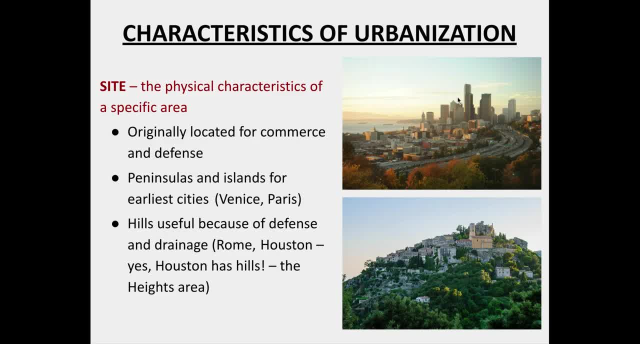 already built into the physical geography. Hills are really, really good for this. You can see the hills in Well, you can see that Houston has hills is what I was looking at, but you can also see the and these images that i grabbed here and, of course, when you're at the top of the hill, you 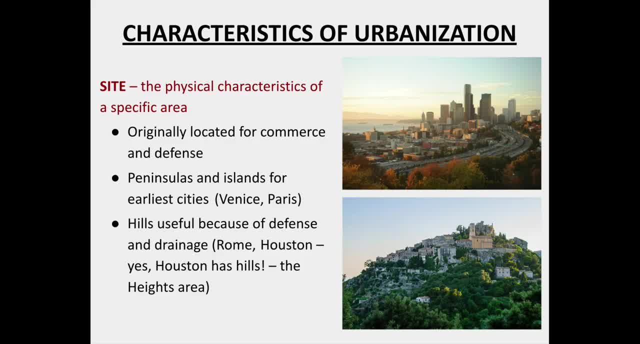 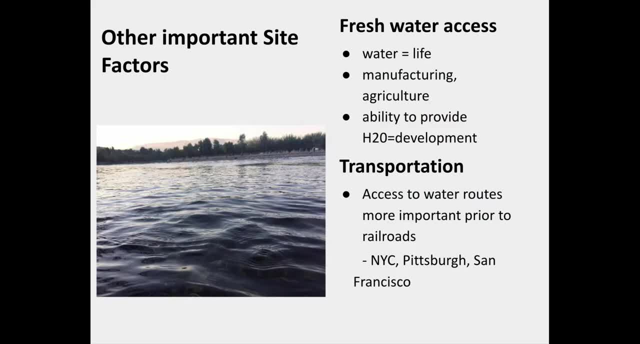 can look it down and see your the invading armies coming in, so it's a kind of an early alert for you. um, so anyway, so that's some of our earliest characteristics. also, don't forget about the importance of water. you should have learned this a very, very long time ago. water is, of course, 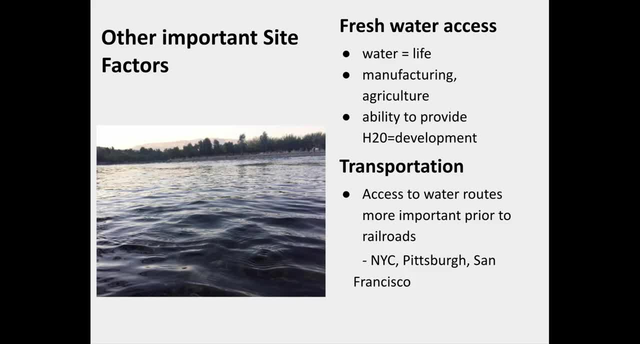 essential for life. but moving forward to the modern era, you have to have access to fresh water or any type of water source for manufacturing, for agricultural production, and it's actually a really great measure of development to look at a country to see how they are able to. 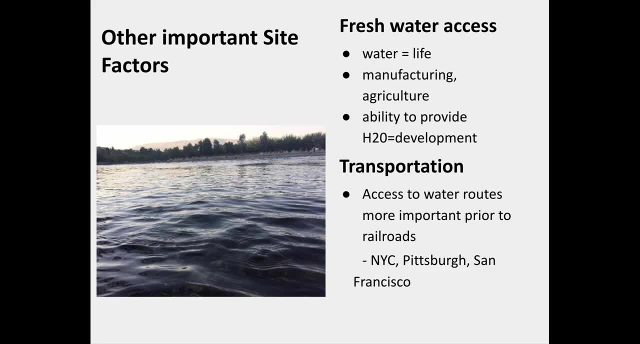 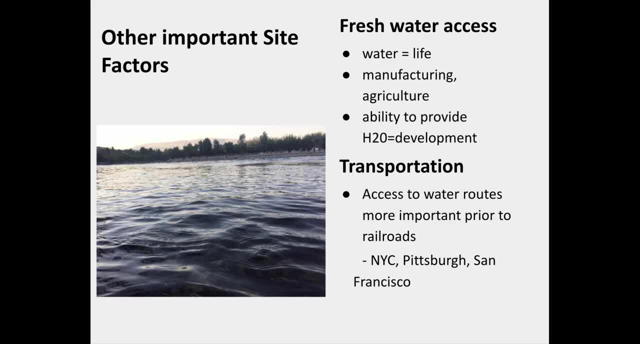 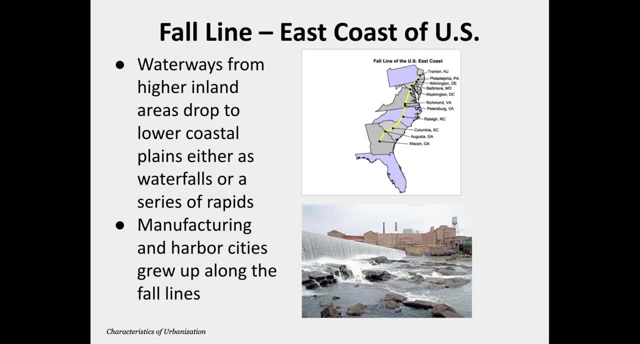 much, much cheaper to ship something via water than it is to ship via rail or air or anything else. uh, one little blurb i want to go ahead and go over with you with regards to vocab: is this concept of fall line. i honestly haven't seen this uh and anything aphd related in a while, but i want to. 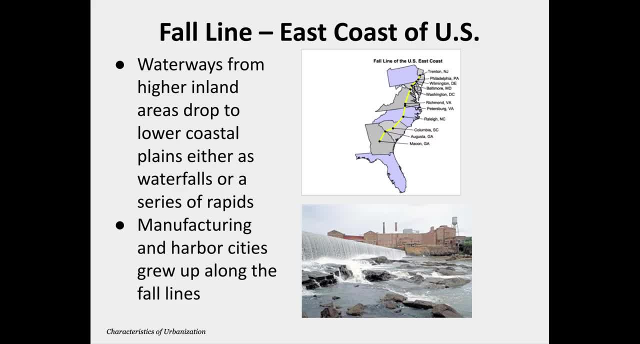 make sure that you guys know what the fall line is. uh, this is along the united states and you could see in that top image there all of the main cities that are located in the fall line. this is just physical geography impacting where cities are located. the fall line is. i don't say literally. 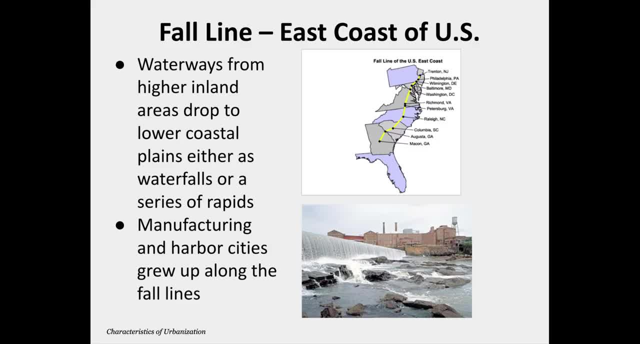 but it's. it's actually a place where you see kind of think of like waterfalls right, where you begin to see this shift in physical geography, uh, in the geology of the region, uh, where you see this change in elevation, and so you tended to see cities that were along the fall line. 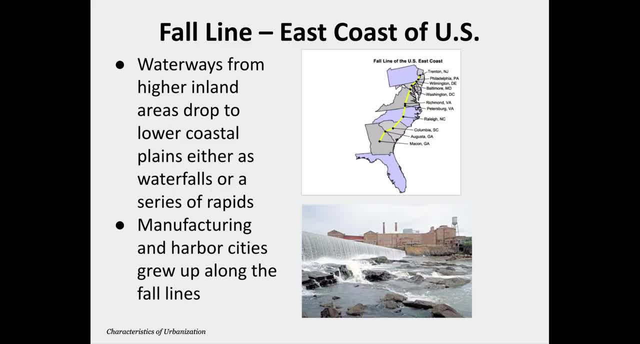 first of all because you can get the energy source from the water falling, but also just because it's really really hard to transport. i mean, look at the. if you can see the waterfall on that little bottom picture there, it's hard to send a ship up that where that. 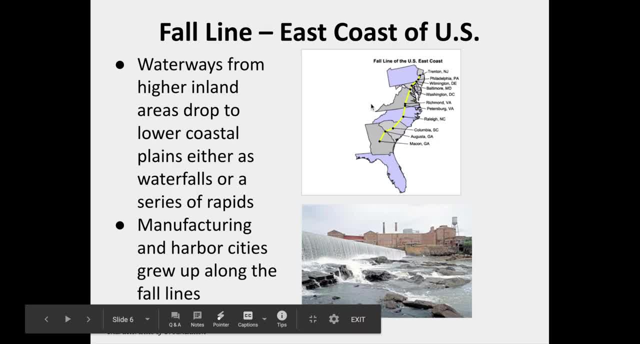 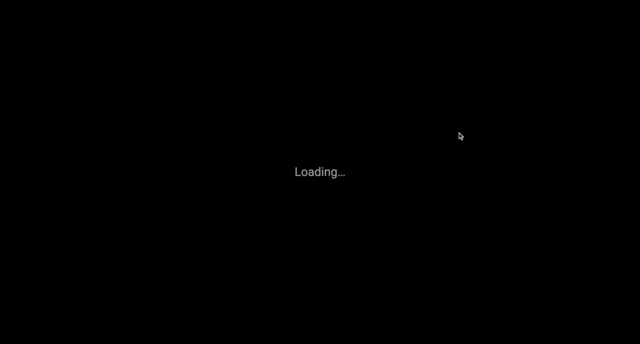 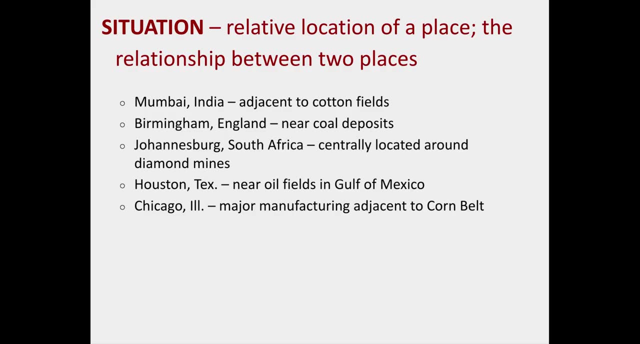 split is in the waterfall line. okay, so those are all site factors. now let's go ahead and look at situation factors. situation factors have to do with the relationship between two regions. so site factors are what's the physical geography of a place. situation factors have to do with the relationship between: 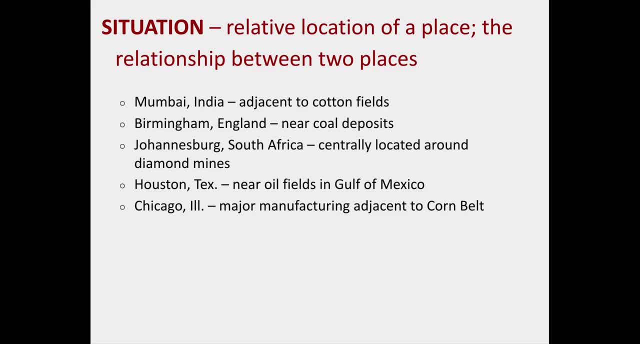 two places. so, for instance, once again i'm in houston and uh, we know that houston is the energy capital of the world and part of that is due to the discovery of uh, and and the use of of oil very, very early. uh, spindle top- you may have heard the story of spindle top, but also 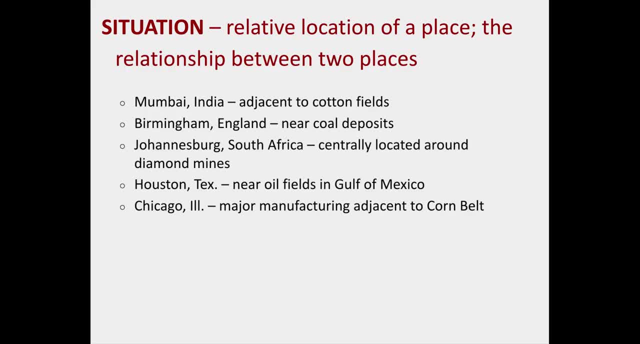 especially recently. uh, we are adjacent to major oil fields in the gulf of mexico. you look at a city like bonita a little bit, but you can see that in the gulf of mexico. i'm not going to go into more detail about those because we're just going to go into the details of where the 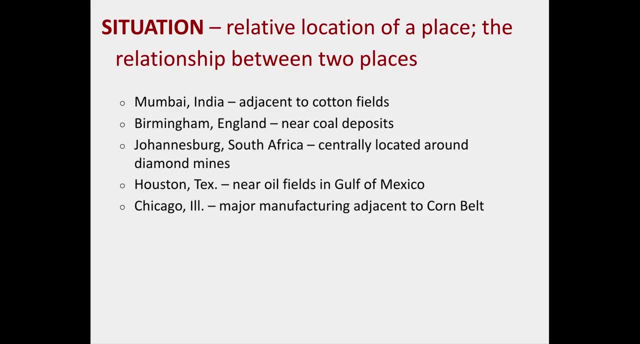 Mumbai, India, big manufacturing hub, And of course those are very close by to the cotton fields that are outside of Mumbai, Birmingham, England. if you recall our discussion of industrialization, that's very, very close by those coal deposits. So, once again, situation. 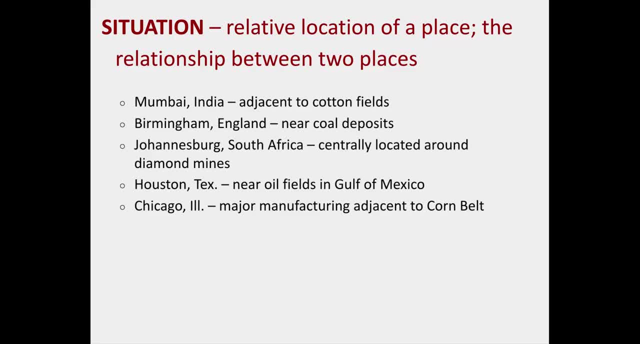 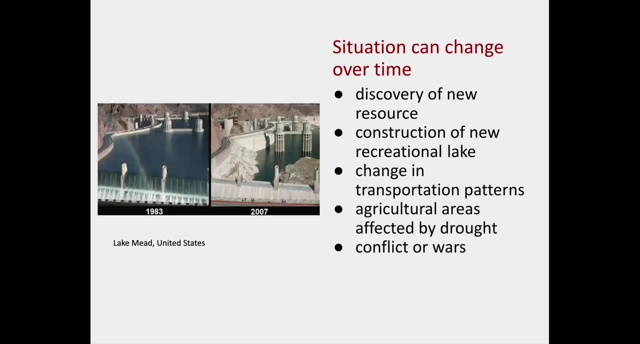 has a lot to do with the success of a city. Think about something someplace like Singapore. The situation of Singapore is fantastic for trade because it's halfway between China and India and all that transit that just kind of passes in between those two regions has to stop in Singapore. 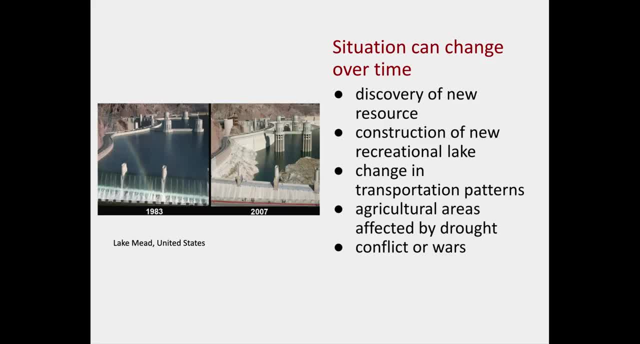 Situation can change over time And I went ahead and I grabbed an image of Lake Mead. You could see the impact of the drought on Lake Mead in the United States. So, with regards to resources, maybe let's say you're looking at a place like Bolivia and you're trying to get 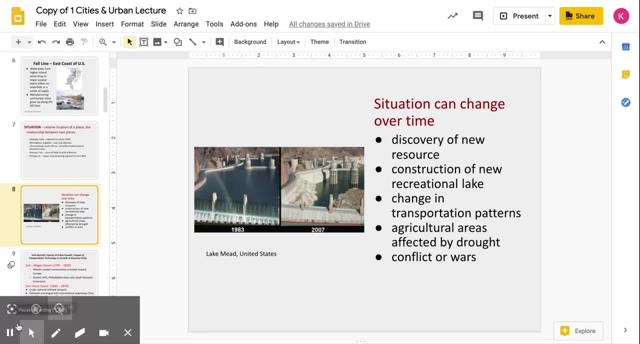 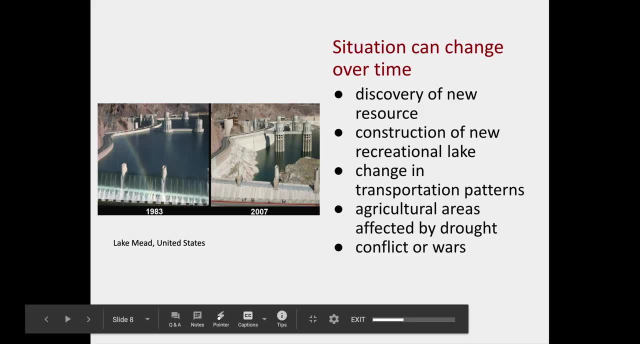 lithium in a place like Bolivia. And then let's say, you find another location of lithium here in the United States. Well, maybe you won't be trading as much with Bolivia anymore if you find lithium here in the US. So just realize that situation, the impact of cities and situation can change over time. 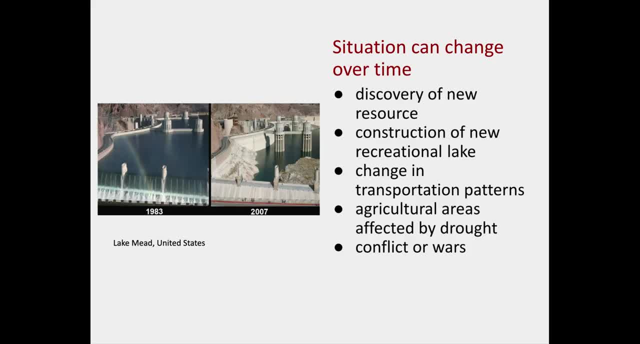 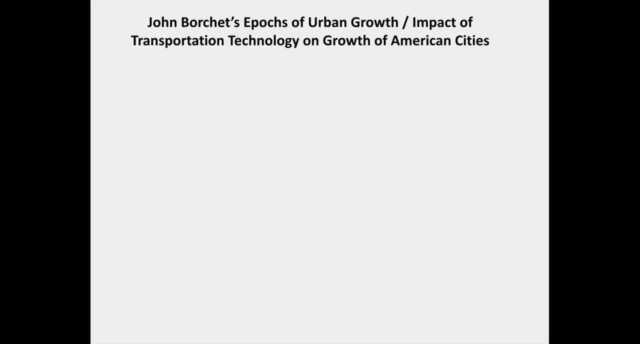 Things like drought, things like wars, transportation pattern changes. Let's think about the South China Sea and China's continued island building in the South China Sea, how that might affect global transit patterns later on down the road. So really good examples of situation changing over time. Okay, Now to change modes completely here. 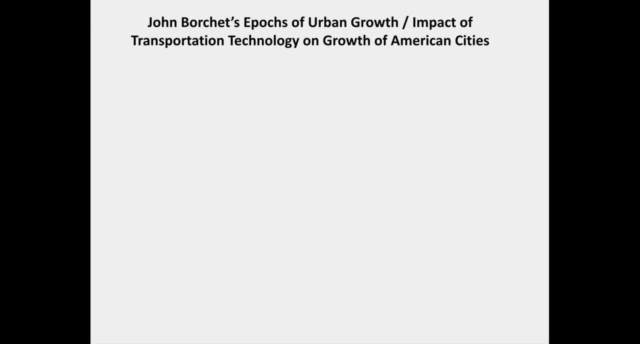 we're going to talk about John Borsche's epics of urban growth, And so, as I'm going through this, I'm going to suggest that you draw something to demonstrate knowledge of these items. So this has to do with this particular section, has to do with how transportation methods and 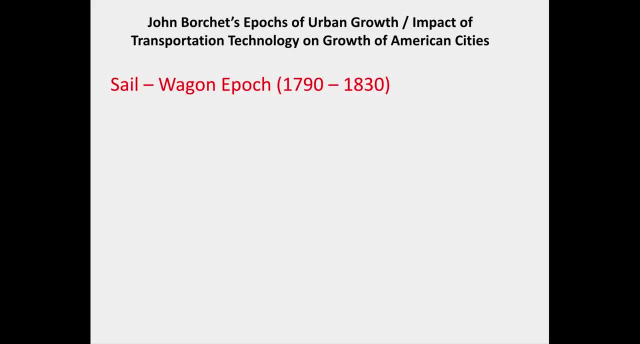 increases in technology have changed how American cities, cities and cities grow over time, And so we're going to go through these one section at a time. The first one is called the sail wagon epic, And of course, look at those dates there, from 1790 to. 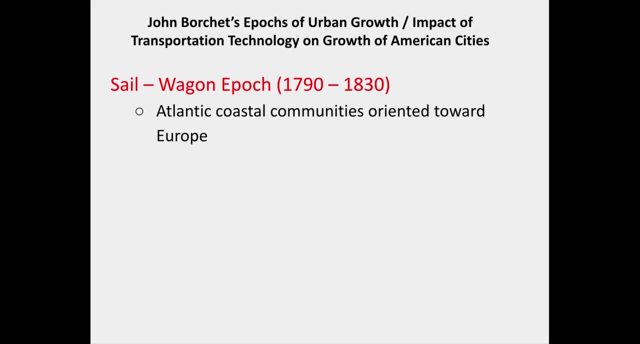 1830.. We're not talking about super high tech here, And so cities, as they're structured, are going to have to deal with the technology that they use for transportation. So we're talking about ships here, right, And of course, wagons. So if I were you, I probably would draw. 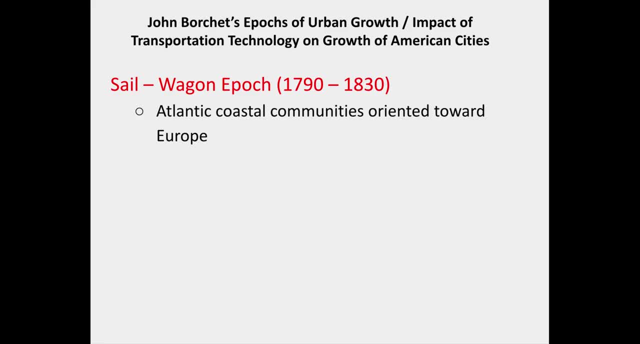 I'd probably stop this for just a second and draw maybe a little boat or a wagon or something to kind of cement in your brain this particular epic. So this is going to focus on the cities in the Northeast of the United States, those 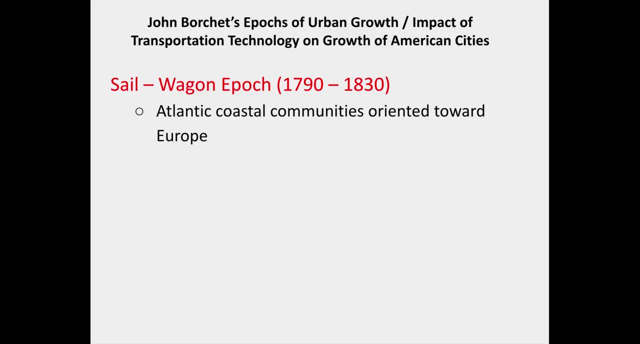 coastal cities and think of colonization and those cities that you studied in colonization. These are going to be all cities that are oriented towards Europe, because that's where trade was happening at the time. So think about cities like Boston and New York and Philadelphia. 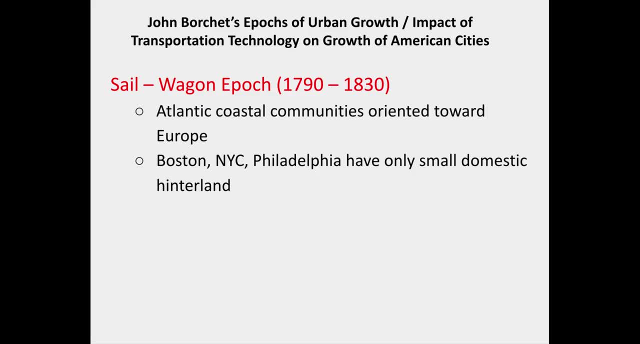 These are cities And, of course, that term hinterland, remember. the hinterland is the surrounding area, It's an area outside of a city. The next epic is what we call the iron horse epic, And if you were thinking what's an iron horse? that would be something like a train, right? And so this is. 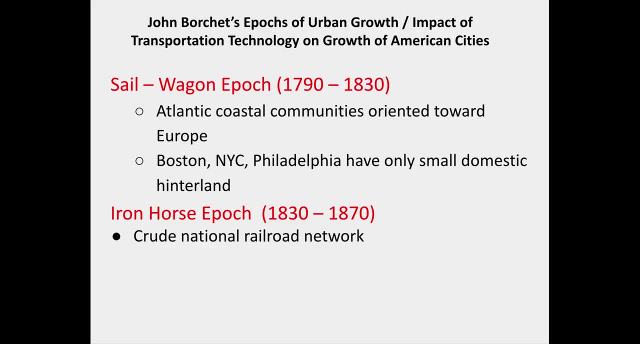 the very beginnings of the rail network that we had in the United States. And, of course, don't forget your US history. who urbanized first? the North urbanized first, of course, And they did that because they had the natural resources, the side factors, the natural resources, the 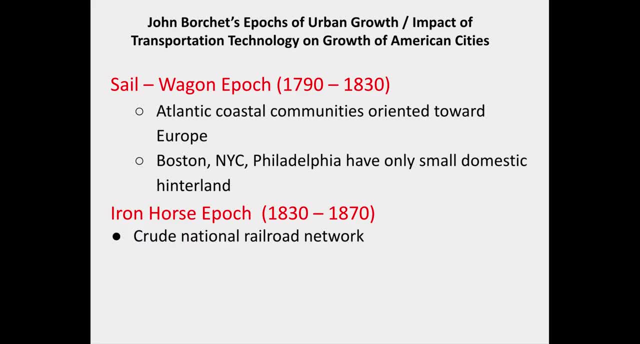 right factors there to be able to urbanize and to create those inventions and utilize those inventions like a rail network. So we're talking about cities in the Northeast, but also moving a bit further West. Think about the Rust Belt area. now These are going to be cities like Chicago. 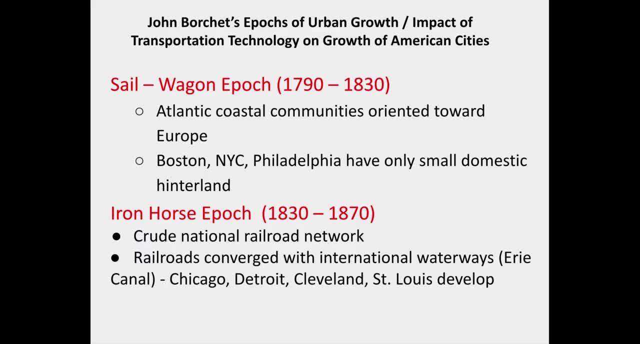 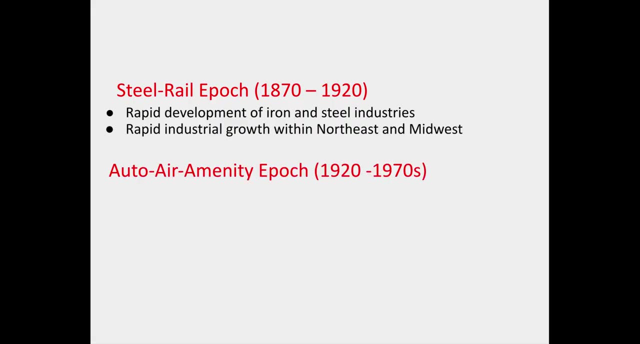 and Detroit, cities along the Ohio River Valley, all cities that were really got the benefit of modern industrialization. Okay, The next one is going to be the steel rail epic, And this runs from 1870 to 1920.. I probably. 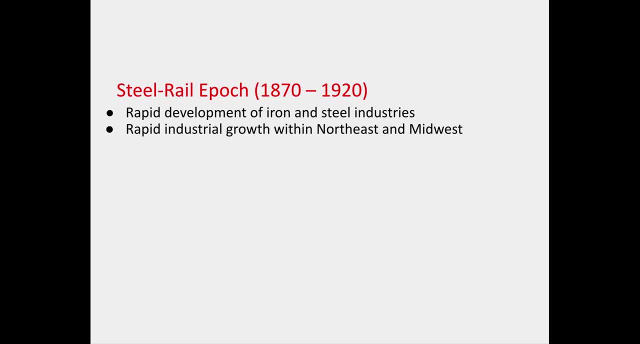 would draw, try and draw, a railroad if I could here some kind of train here. But this is really showing the profusion, the spread of the rail network. And of course, once again, notice this is further North here, right, And think about those cities during this particular time. Think. about cities like Detroit and Chicago And of course, this is the steel rail epic And this is really showing the profusion, the spread of the rail network. And of course, once again, notice this is further North here, right- And think about those cities during this particular time. Think. 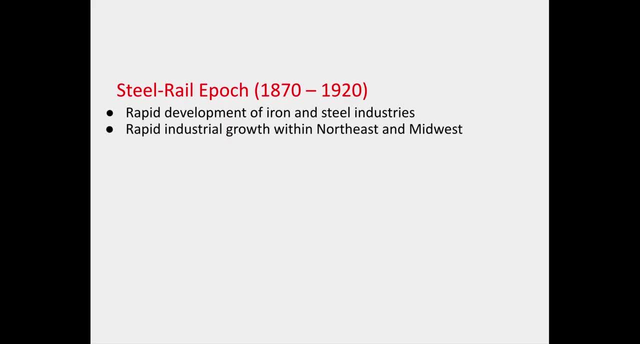 about those cities during this particular time And, of course, once again notice this is really moving cities And then of course, moving a little bit further South from that, but still kind of staying in the Northeast and moving towards the Midwest. We had definitely haven't. 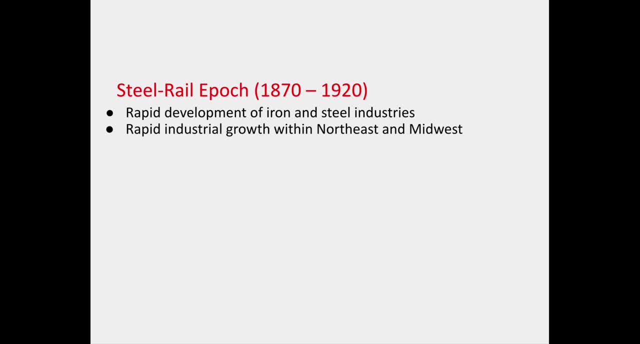 gone anywhere below the Mason liksom Dixon line yet. That will be soon, but these are going to be cities that are part of that steel rail epic. The next epic will be the auto air amenity epic, and this runs from the 1920s to the 1970s And, of course, at this point in time, your technology. 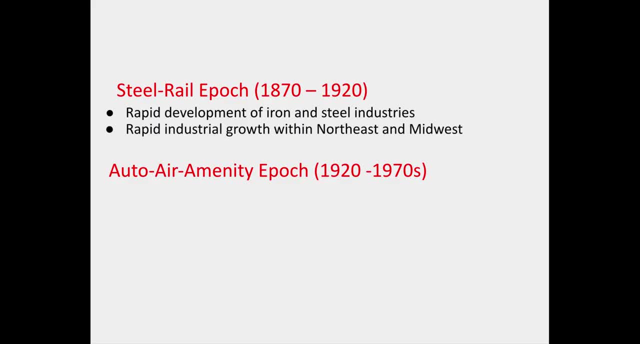 change will have an impact on the city, So we're talking about cities that are part of the steel. Changes are pretty substantial now, So we start with automobiles in the early 1920s, And then, of course, we push through to the 1970s. 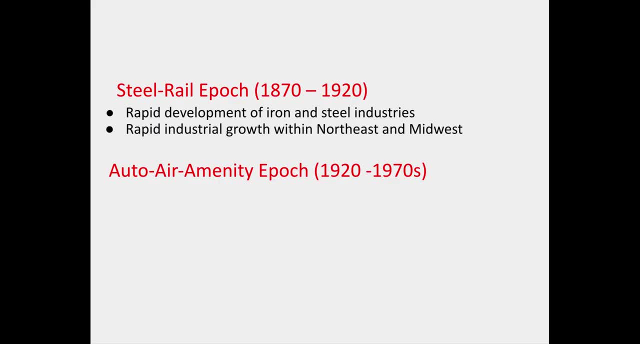 And this begins to show how cities during this time were really impacted by the growth of the automobile. So you begin to see throughout the United States, this really complex network of transportation. So think about, if you've seen the movie Cars, think about the impact of Route 66 that the interstate highway system had on Route 66.. 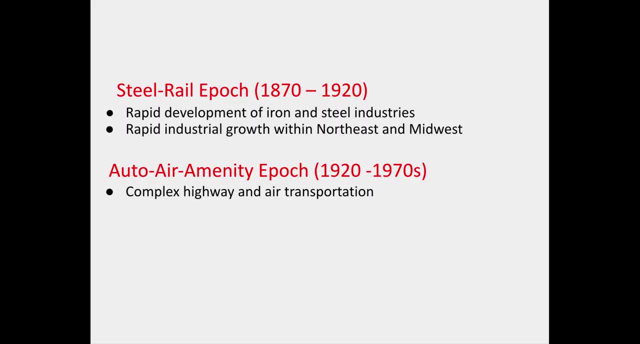 So cities that were formed along that during the time and then how they shifted and changed with the interstate highway system that was created. Also, with these improved amenities and speed of people transporting themselves and goods and products, you also had increased suburban demand. So think about a city like Los Angeles or think about a city like Houston. 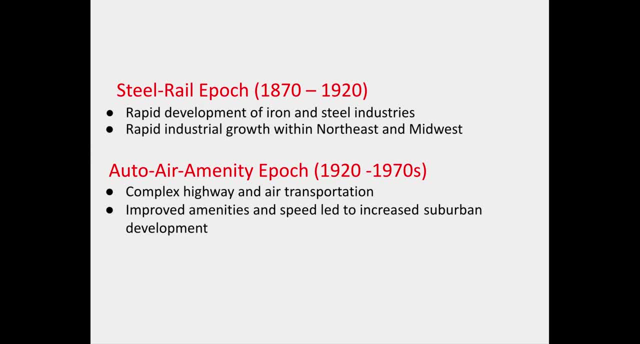 Once again, these are cities that grew up after the advent of the automobile, And that's why these cities are so so spread out. Houston is the size of Rhode Island, And the reason why is because this city was pretty much came to fruition. 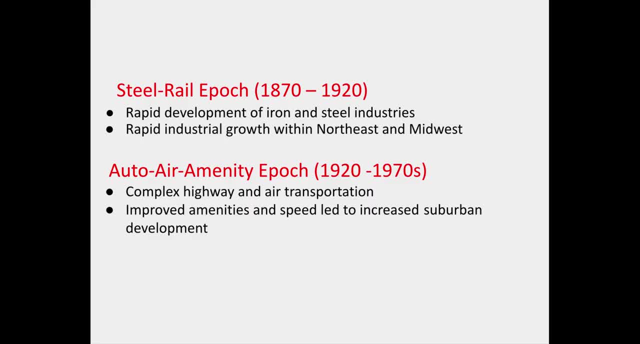 Even though Houston has been around for a while- modern Houston came about really in the 1940s and 1950s. Also this term Sunbelt remember. so the Rust Belt is the area that runs from the northeast all the way kind of through to, and through Pennsylvania, Ohio, really all the way over into Illinois. 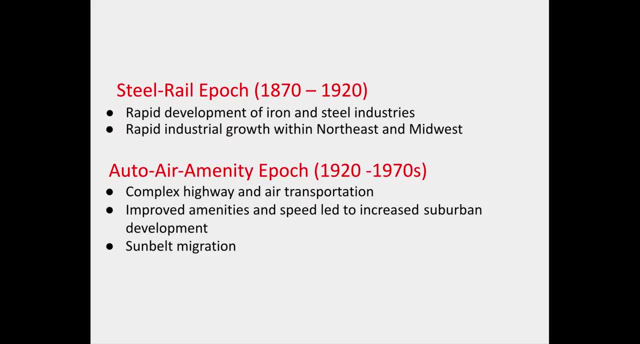 The Sunbelt region runs from Georgia kind of along Florida, Alabama, Mississippi, Texas, all the way through over to California And these are all going to be regions where your cities that were again, I don't want to say growing up, but being formed during this time. 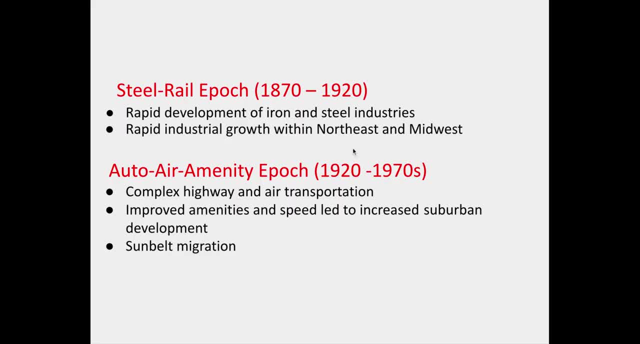 these are cities that came about after the advent of the automobile. One other thing to consider about the Sunbelt migration is- and I don't really have it on here- a bullet point, for it was the impact of air conditioning. Those of you that live in the South you know that summertime is miserable here.